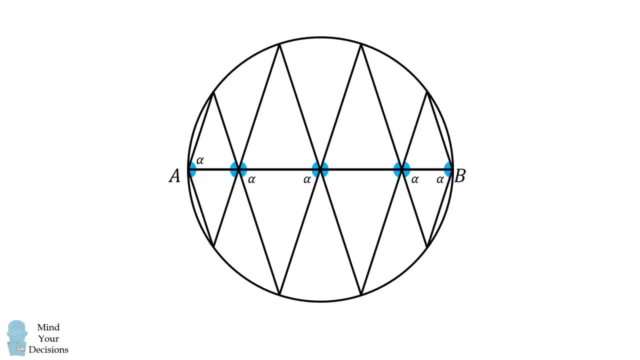 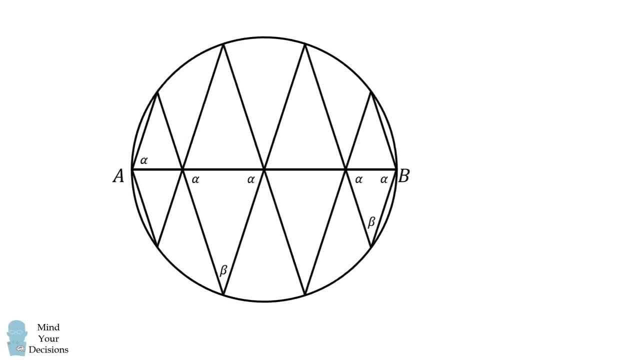 Next we'll label some of these equal angles as alpha, Label the remaining angle in this triangle as beta. From here we're going to consider the measure of the arc BC. We'll calculate it in two ways. First, CAB is an inscribed angle of the circle with an angle equal to alpha. 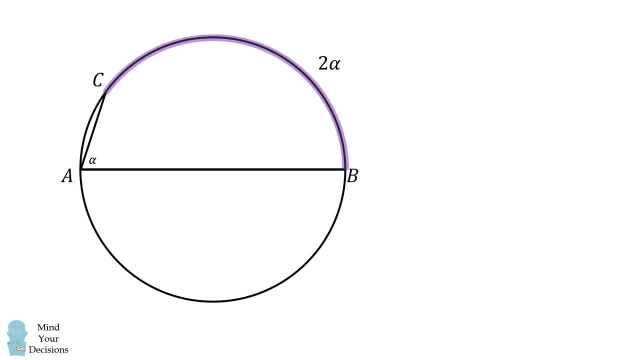 Therefore, BC will be equal to 2 alpha. We will calculate BC in one more way. Notice: we have two inscribed angles, each of which is equal to beta. So this arc will have a measure equal to 2 beta and this arc will have a measure equal to 2 beta. 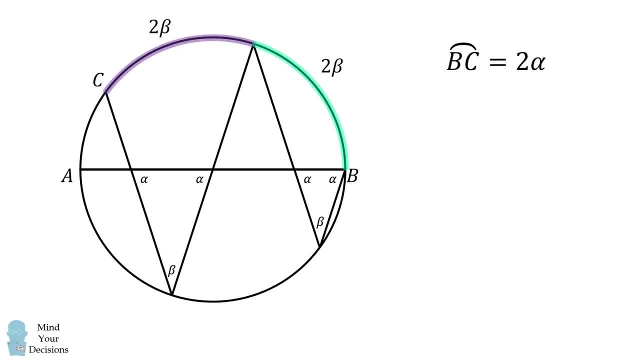 Therefore, BC will have a measure that's equal to 4 beta. We thus have: BC is equal to 2 alpha, which is equal to 4 beta, which means that 2 alpha is equal to 4 beta. We'll divide both sides of this equation by 4 to solve for beta. 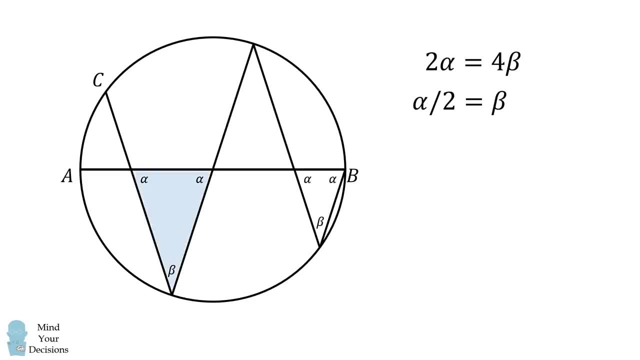 Beta is equal to alpha over 2.. Now we have a triangle where two of its angles are equal to alpha and one angle is equal to beta. Thus we have 2 alpha plus beta is equal to 180 degrees. We can substitute for beta and then we can solve this equation for alpha. 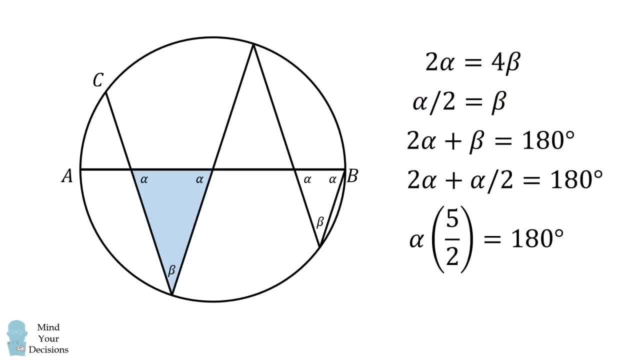 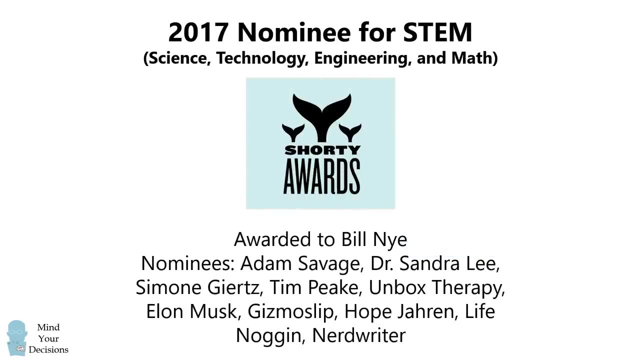 We get: alpha multiplied by 5 over 2 is equal to 180.. We'll multiply both sides of the equation by 2 over 5, and thus we have: alpha is equal to 72 degrees, And that's our answer. Thanks for making us one of the best communities on YouTube.